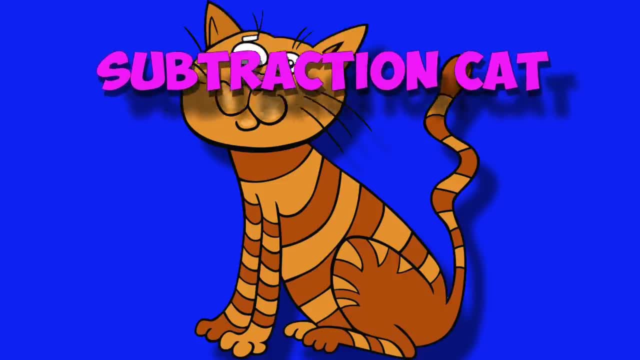 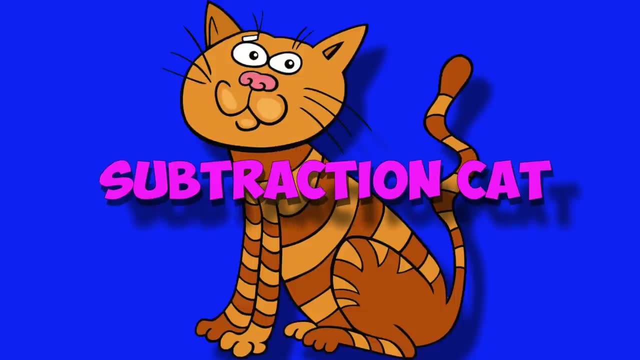 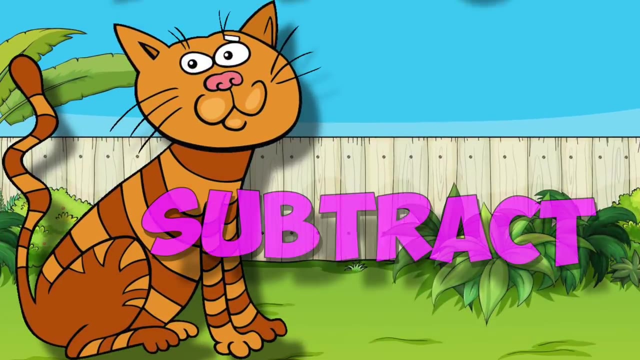 Subtraction Cat: What's up with that? Don't eat the mice, or you might get fat. Subtraction Cat: What's up with that? Don't eat the mice or you might get fat. There once was a cat who liked to subtract, who liked making things go away. 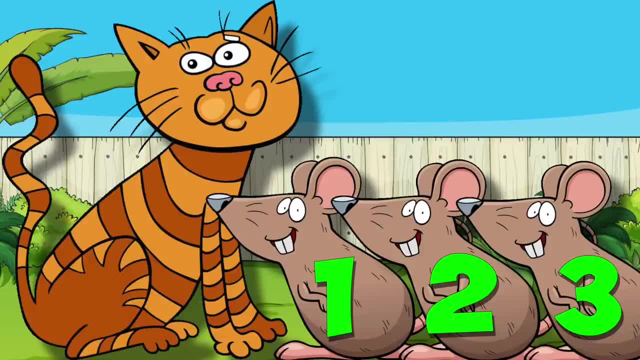 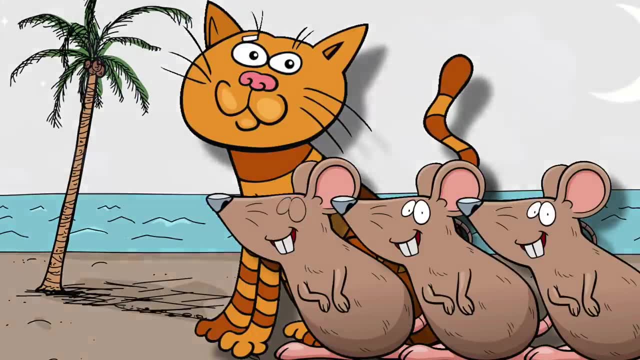 One day she spied mice and she treated them nice and asked three of them to stay put and play. They played in the park and out at the beach. They played as the day turned to night, But when the mice were distracted, the cat then subtracted. 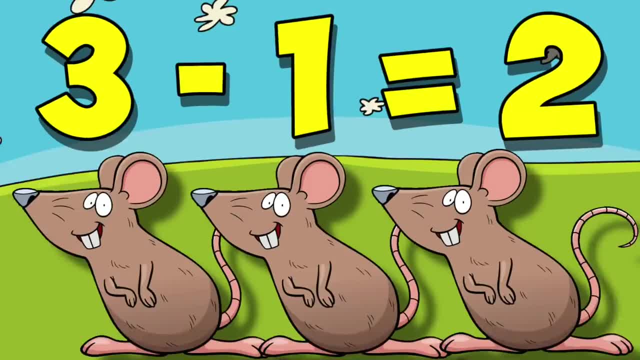 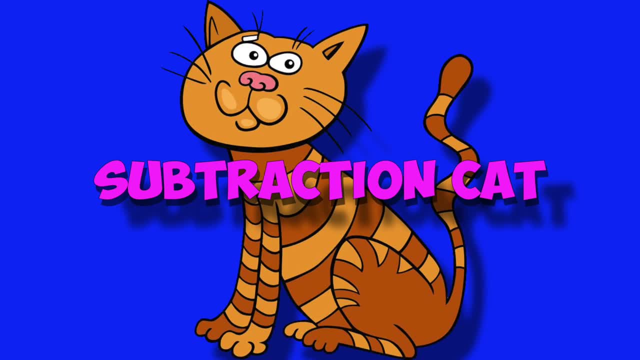 Three minus one was all right. Three minus one is equal to two. Now it's time for everyone to sing. Subtraction Cat- What's up with that? Don't eat the mice or you might get fat. Subtraction Cat- What's up with that? 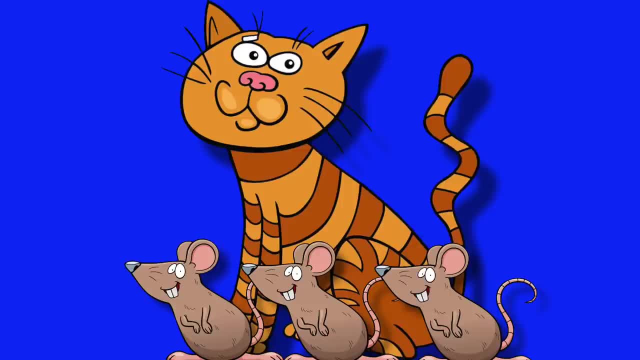 Don't eat the mice or you might get fat. Subtraction: Cat. What's up with that? Don't eat the mice or you might get fat. Well, just two mice remained to play cat and mouse games, and they had so much cat and mouse fun. 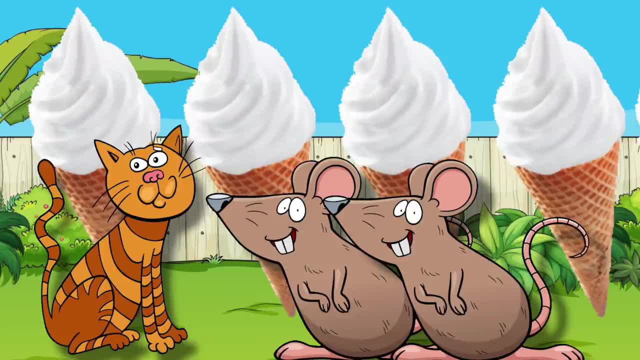 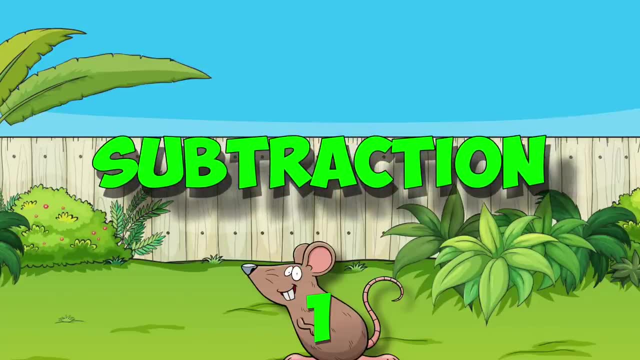 They went off to the zoo and to the children's museum. They enjoyed ice cream in the hot sun, But the thing that occurred- well, subtraction is the word cost. a number of mice was then one. Just one mouse remained to play cat and mouse games. 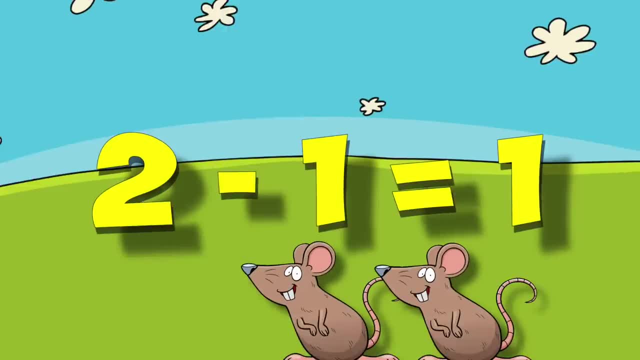 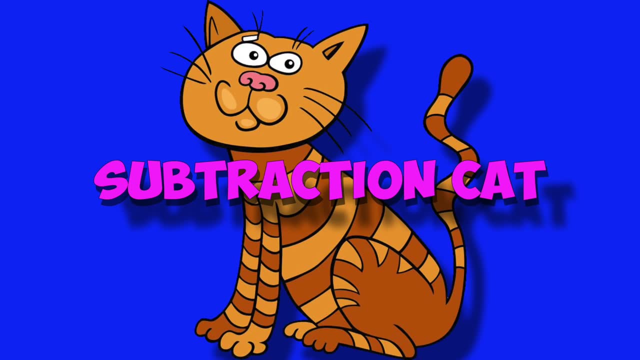 Subtraction still seemed like good fun. Two minus one minus one is equal to one. Now it's time for everyone to sing Subtraction Cat. What's up with that? Don't eat the mice or you might get fat. Subtraction Cat. 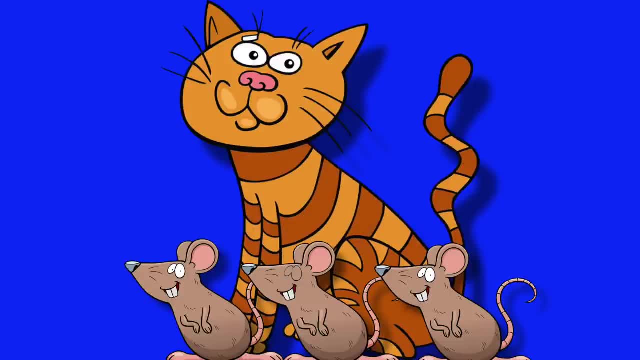 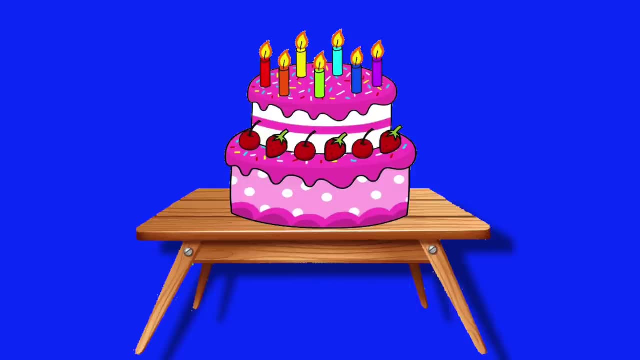 What's up with that? Don't eat the mice or you might get fat. The cat and the third mouse? well, they painted the house, They baked cakes and some other sweet snacks, They swam in the creek and they played hide and seek. 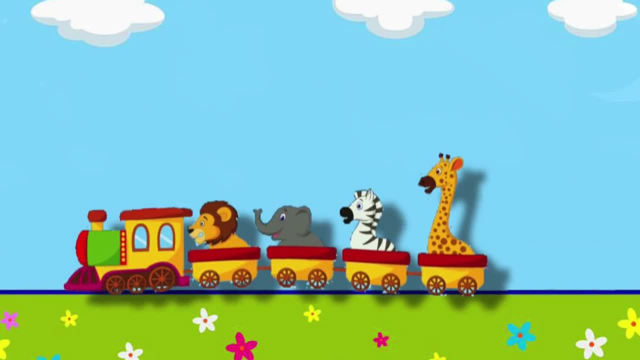 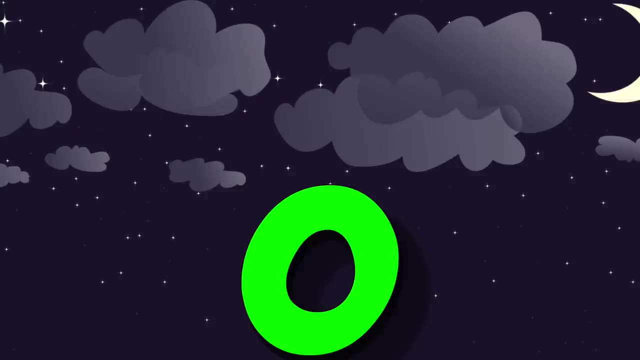 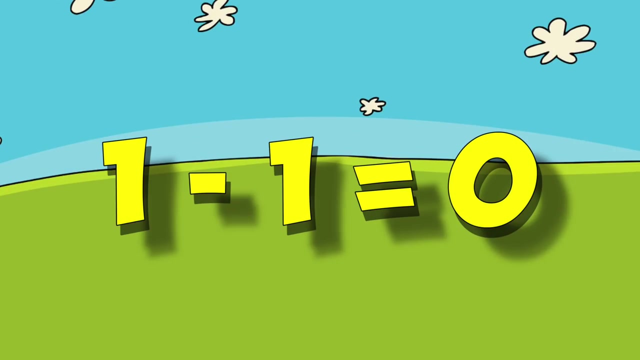 and they set up toy railroad tracks. But at the end of the day, well, what could we say? Cat got right into math action. Now, what had Cat done? Because now there were none, Zero had been made by subtraction. One minus one is equal to zero.